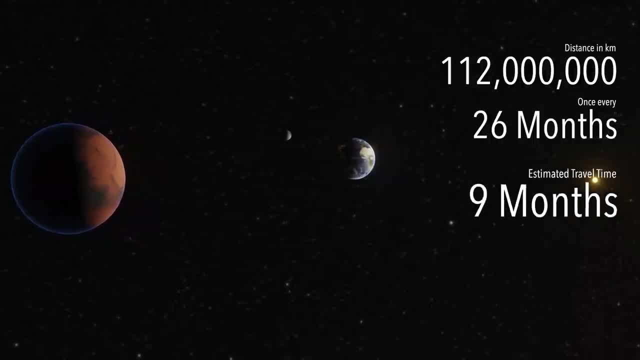 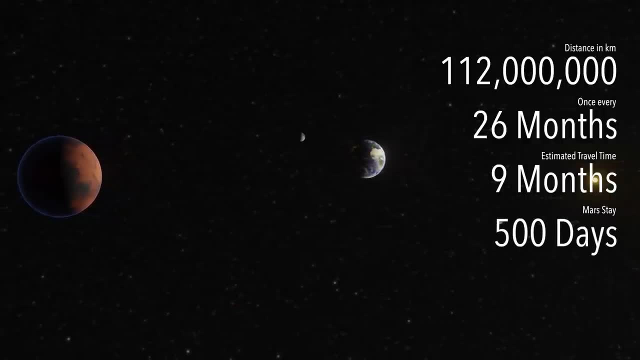 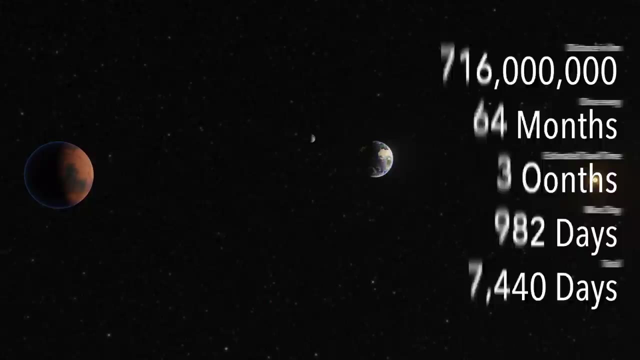 When the time comes. it takes about nine months to reach Mars. at the lowest energy requirements, A round trip would involve 500 days waiting period on Mars for the next window to travel back to Earth, totaling 1,040 days. Throughout the trip, astronauts are expected to receive 0.66 sieverts of radiation exposure. 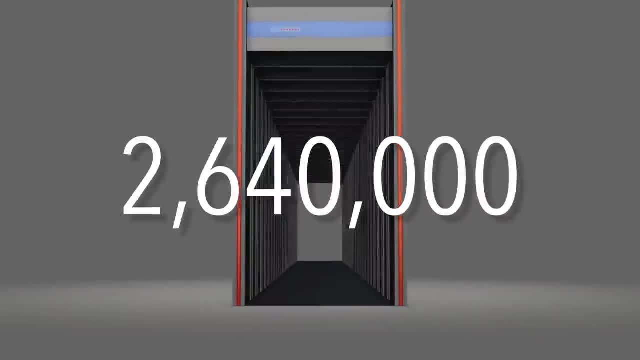 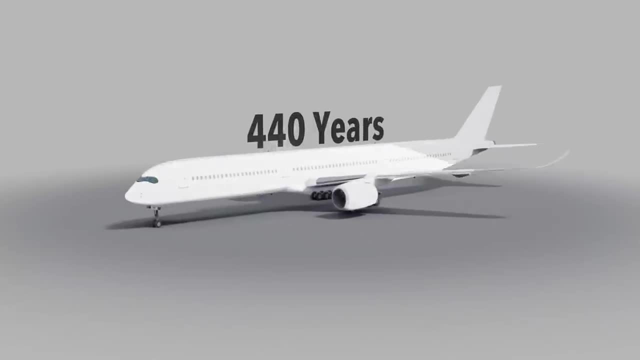 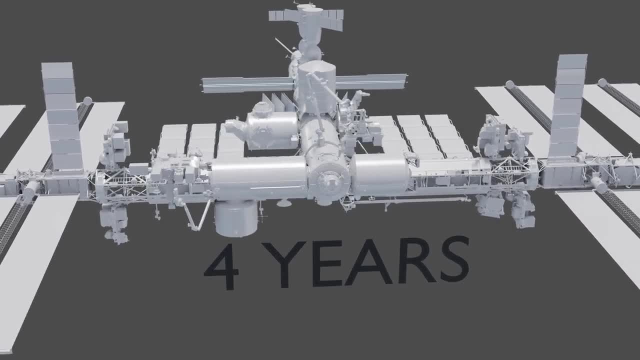 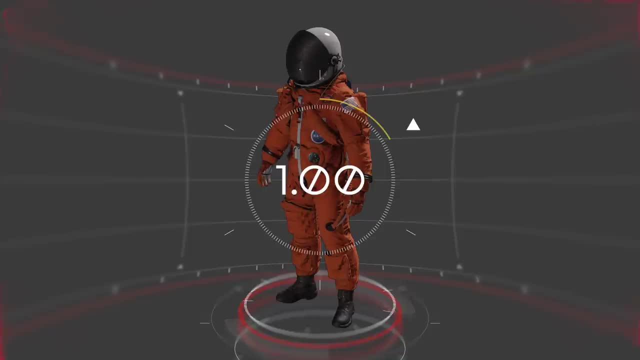 2.6 million seatbelts, or living on board the ISS for four years straight. One sievert is the maximum dose allowed by NASA for astronauts during their entire career. Anything more and damage is irreversible. Five sieverts and you're dead. On top of that, the effects of zero-g force on the human body gets worse the longer you stay in space. Six months is when you really start to see the problem. Your arteries become rigid as though you've aged 20 years, along with blood flow problems. 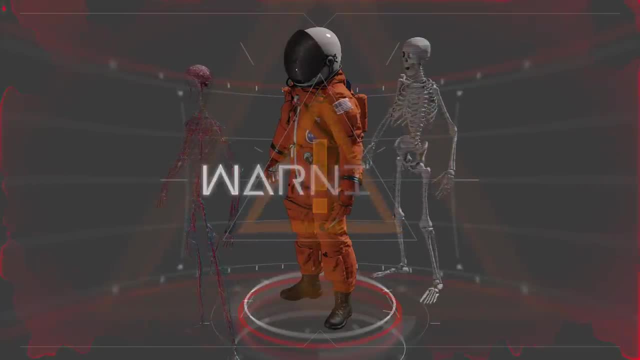 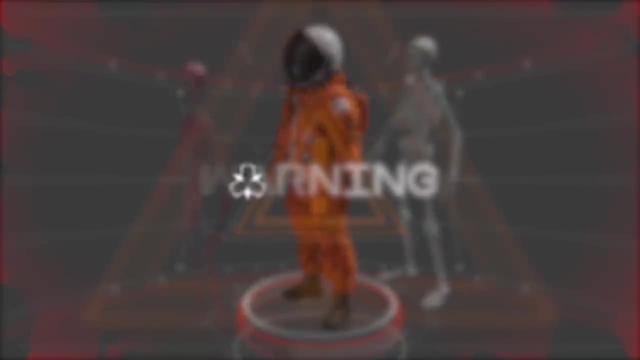 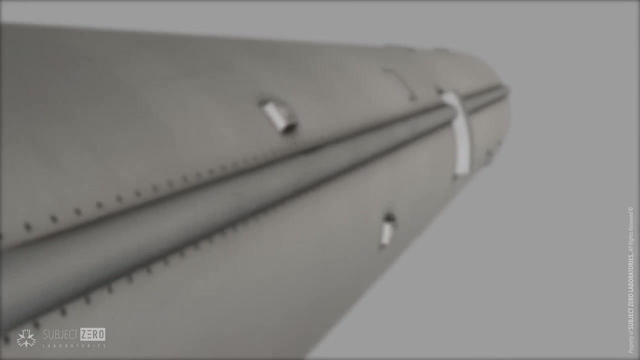 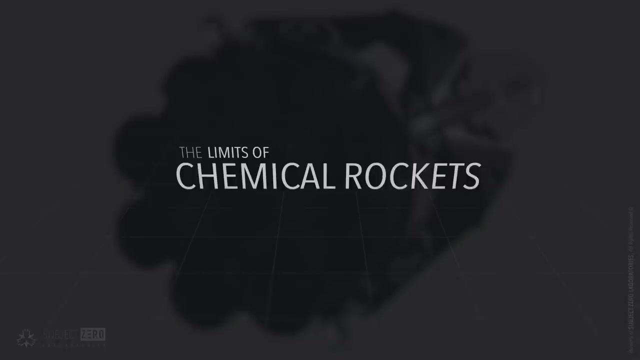 bone density loss and eyesight impairment. Traveling to Mars is definitely one hell of a trip. Hello everyone. Subject: Zero here. For decades we've relied on chemical rockets to take us to space. They work fine for relatively short distances, like going to the moon. 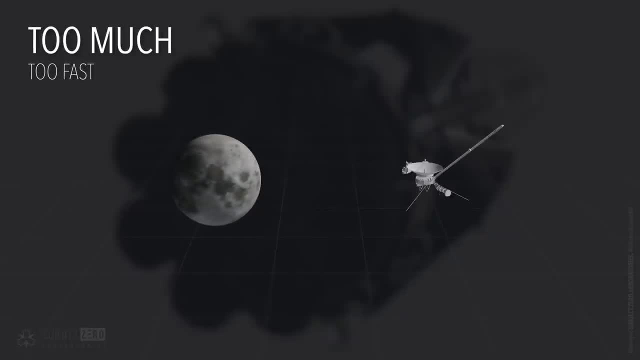 delivering satellites to orbit or even humans to the International Space Station, As we envision going beyond. chemical rockets become more of a limitation than anything else. It all comes down to the maximum exhaust velocity that can be achieved by a chemical reaction. Rocket engines work with basic principles such as Newton's third law of 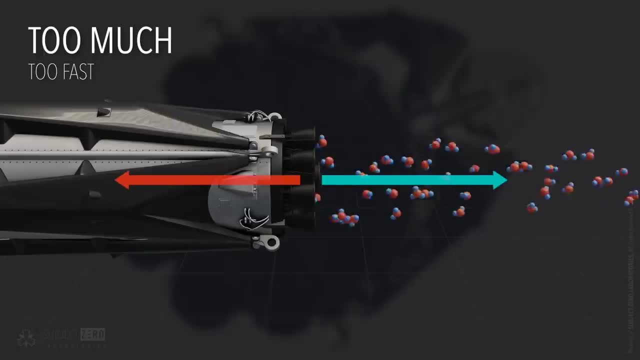 motion. For every rocket that is launched into space, there is a certain amount of energy that is produced each time. In every action, there is an equal and opposite reaction. Chemical rockets use hot gases that are created by chemical combustion, such as hydrogen and oxygen. 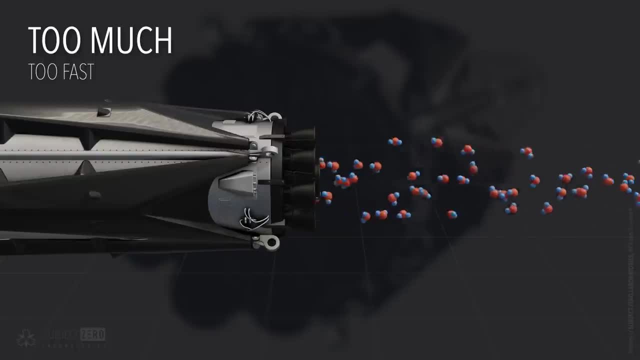 to create thrust. A way to visualize this would be with a shotgun, where instead of bullets, we use molecules. If we take into account the mass of these molecular bullets and their velocities, we can calculate thrust using the following equation: Where F is the thrust measured in. 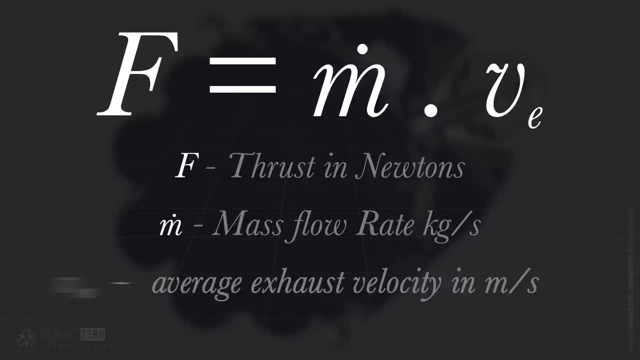 m. dot is the mass flow rate in kilograms per second, and v is the average exhaust velocity in meters per second. What this equation shows is that to maintain thrust constant, we can either increase mass flow rate and decrease the average exhaust velocity, or the opposite. 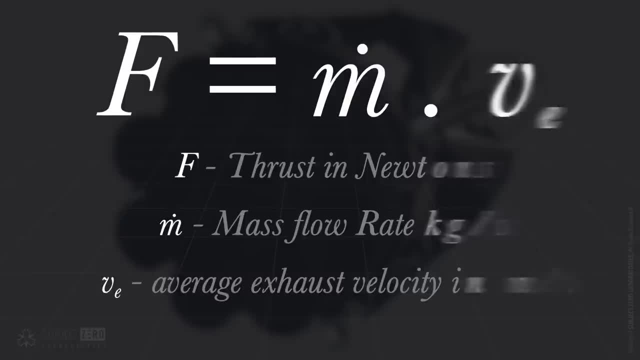 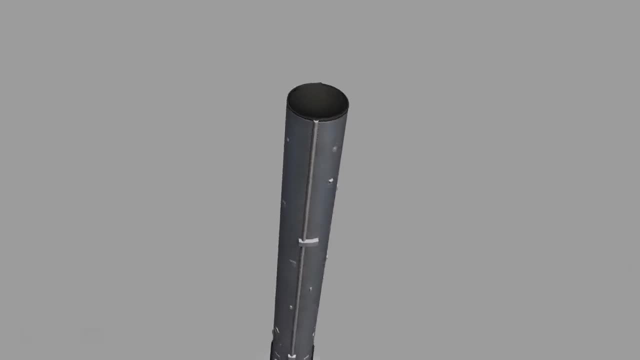 To be successful, good thrust levels are required while consuming the least amount of fuel possible. Chemical rocket limitations can be seen in current technology. The SpaceX Falcon 9, first stage, can produce 7.6 million newtons of thrust. Using the thrust equation, we can calculate how much mass is being expelled by the first. 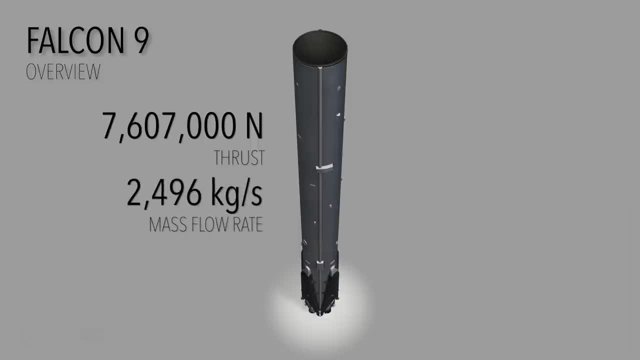 stage of the rocket on average About 2,496 kilograms per second, which depletes the first stage in only 174 seconds. That is enough to take 22,800 kilograms of payload to low Earth orbit, or 8,300 kilograms. 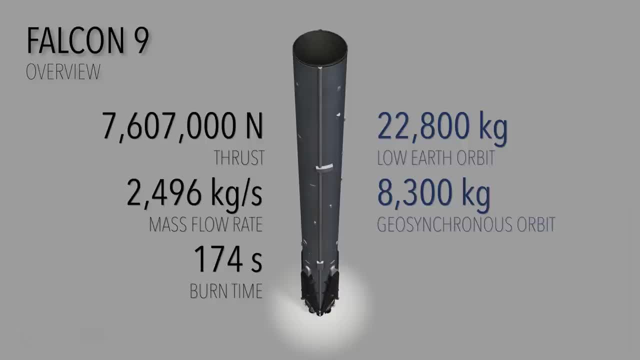 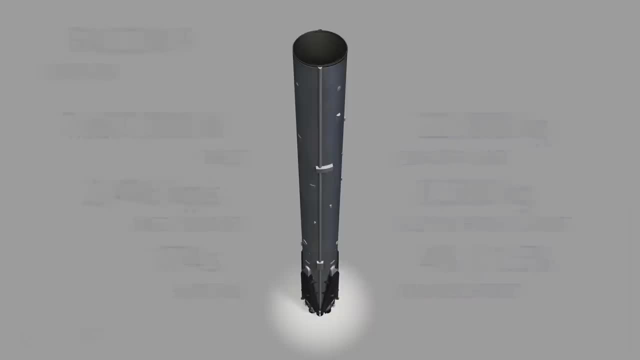 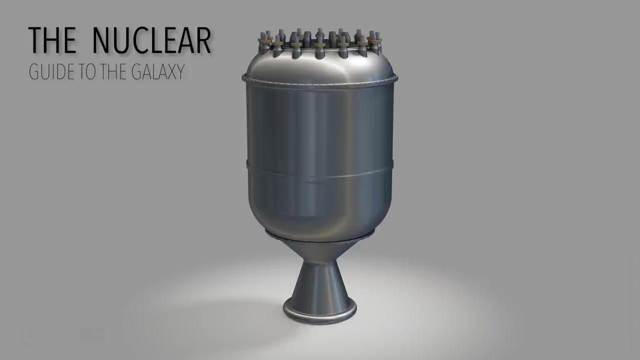 to geosynchronous orbit. Sounds like a lot of cargo, but that is only a fraction of the total weight of the rocket, About 4% and 1.5%. High exhaust velocity is key for performance, since you can accomplish space missions with. 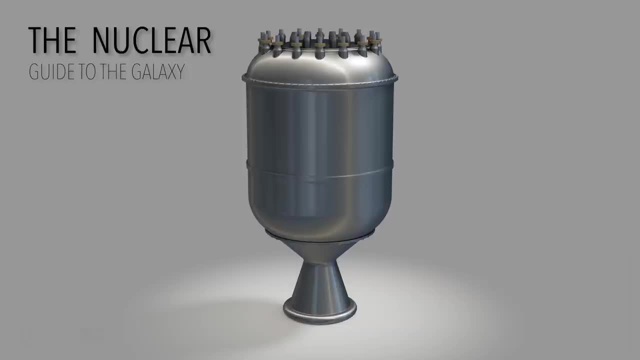 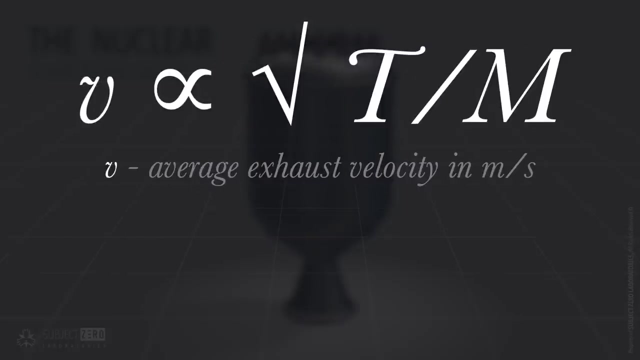 less propellant, Therefore less fuel, lighter spaceship. The problem is: how do you increase exhaust velocity? Nuclear propulsion success can be derived by one simplified thermodynamic equation for exhaust velocity. Exhaust velocity is proportional to the square root of the absolute temperature divided by 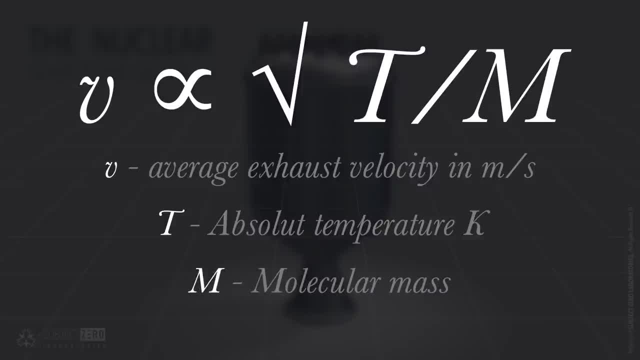 the molecular mass. What this equation shows is that the lighter the molecular element, the higher the exhaust velocity will be. thus hydrogen becomes the fuel of choice for nuclear propulsion. The big difference here is that chemical rockets rely on the energy available from the chemical 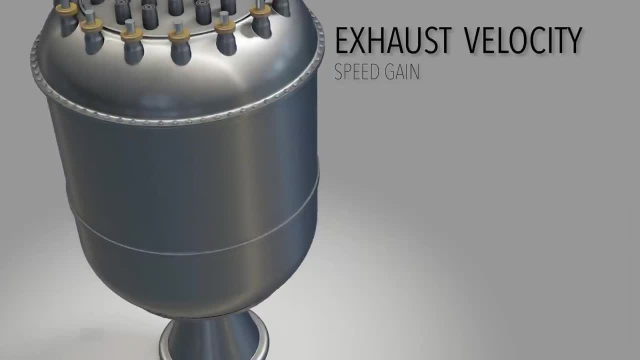 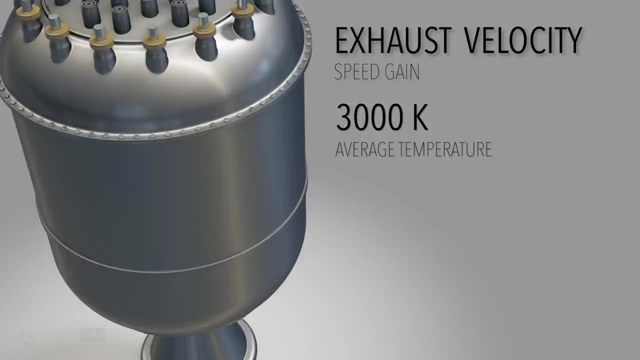 reaction itself. To demonstrate this, let's use the average temperature of most rocket engines. The average temperature of most rocket engines depends on the temperature of the rocket. If we consider the speed of water expelled from the main engine of the space shuttle orbiter m equals 18,, we will have a gain of almost three times the speed with hydrogen. 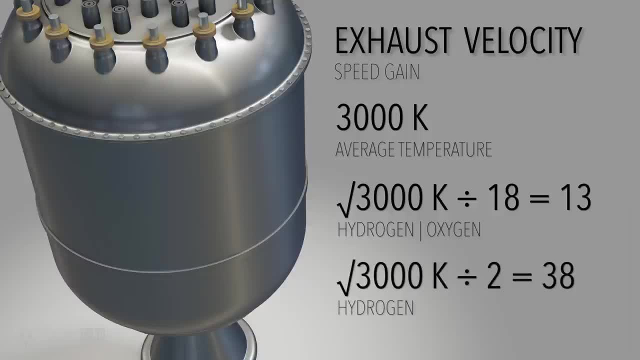 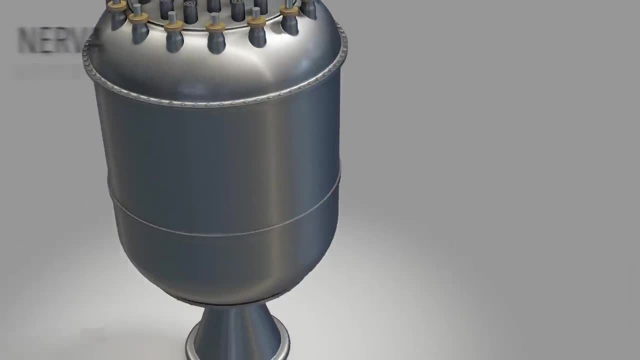 m equals 2.. However, increasing exhaust velocity comes at a cost. Where can we get the required power from? In the late 1960s, early 1970s, nuclear thermal rockets were fully developed. They were designed to be able to produce a lot of energy. 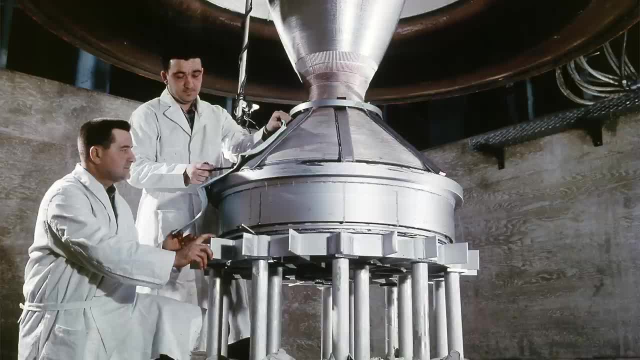 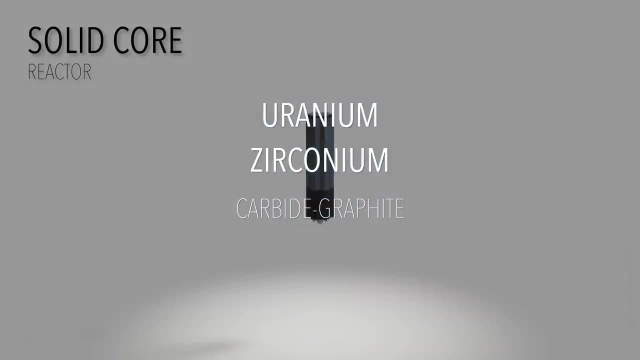 They were fully developed and tested under programs such as the Nuclear Engine for Rocket Vehicle applications, aka NERVA. This program was just one of the two categories that study nuclear propulsion. In this project, they developed a solid core reactor based on uranium zirconium carbide. 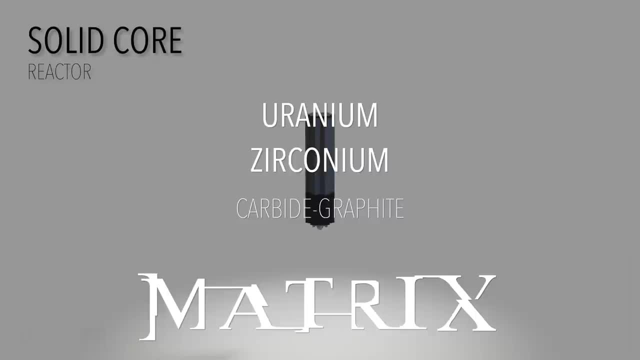 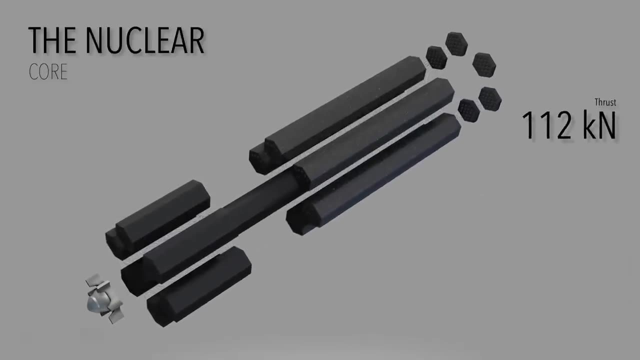 graphite matrix. There were four main configurations tested with increased thrust levels. The largest NERVA-derived engine produced approximately 112 kilonewtons per second. The largest NERVA-derived engine produced approximately 112 kilonewtons per second. The largest NERVA-derived engine produced approximately 112 kilonewtons per second. 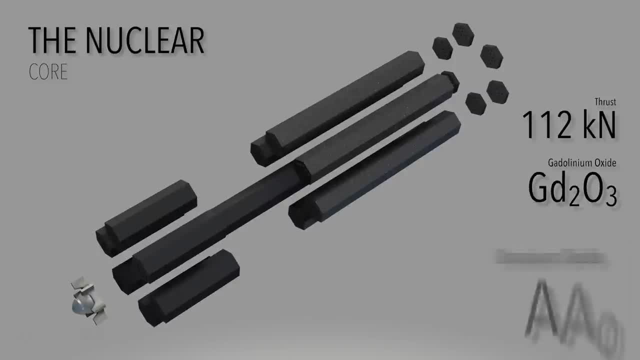 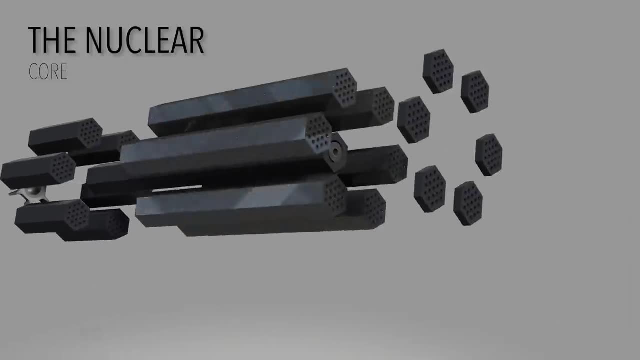 The largest needed fuel is the fuel element of 235 kilonewtons. The fuel element was a complex mix of gundolinium oxide and uranium oxide particles distributed along a tungsten matrix. Each fuel element was hexagonal in shape, with 19 coolant passages. 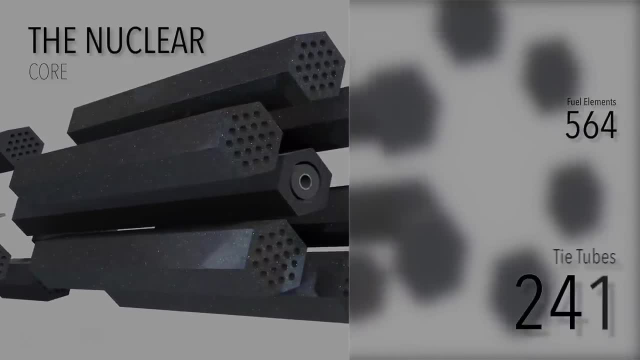 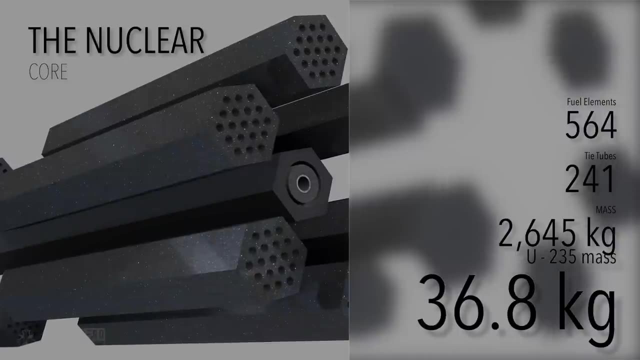 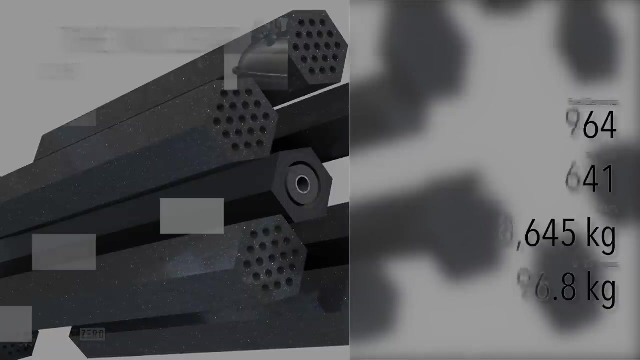 A total of 564 fuel elements and 241 tide tubes were used, with a total mass of 2645 kilograms, containing 36.8 kilograms of uranium-235.. 555 megawatts. Just like in conventional rocket engines, the nozzle is cooled by hydrogen. that 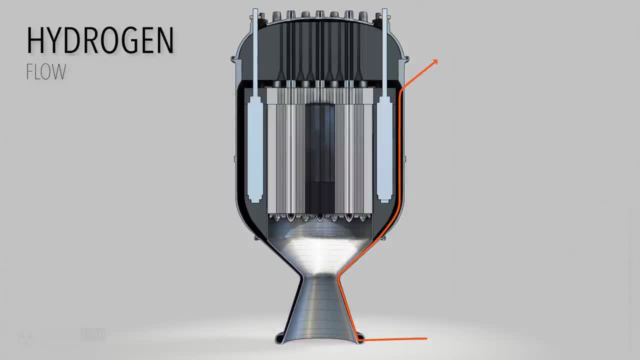 comes in through the inlet valve. It is then transported upwards to the outside of the reactor, towards turbo pumps that increase its pressure. At the same time, a second flow of hydrogen is pumped into the tie tubes, which further increase temperature and pressure. This flow is added to. 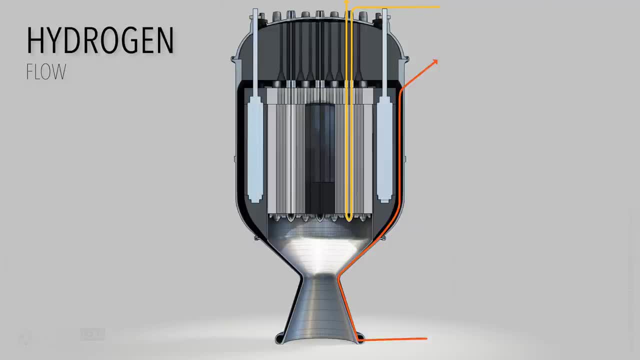 flow number one, and it's directed towards the second set of turbo pumps. In this last phase, hydrogen goes back to the core, passing through the fuel elements, where it experiences the largest increase in temperature, from 367 kelvin to 2794, with a mass flow rate of 12.6 kilograms per second. 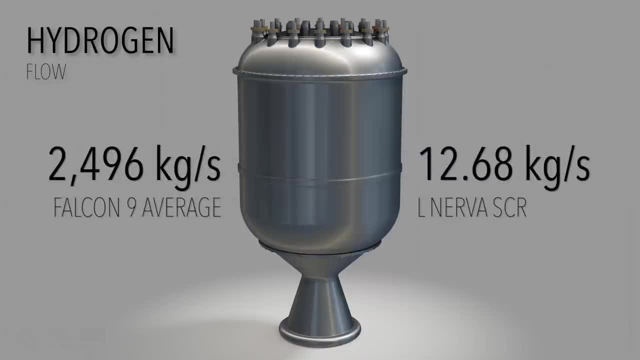 A quick comparison with the average flow rate of the Falcon 9 rocket at 2496 kilograms per second, and it makes it easy for you to understand the difference between the two. First of all, it makes it easy for us to understand why nuclear is the best choice for space travel. 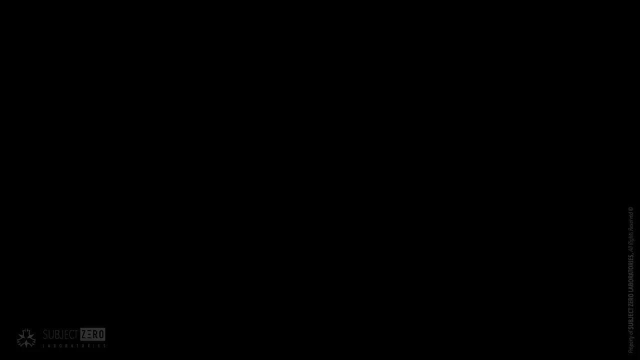 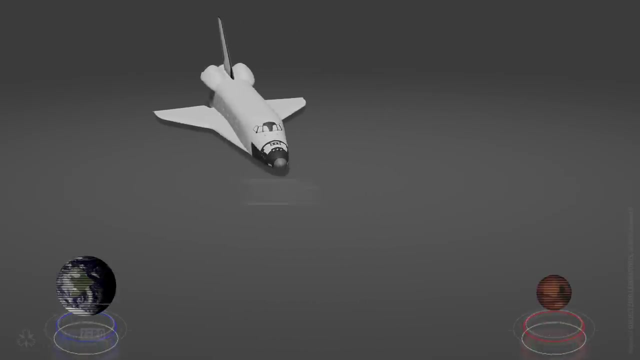 not lifting large payloads into space? Why should we consider the nuclear option To travel to Mars? I am considering a ship that is 220 tons, plus the necessary fuel mass to accelerate the ship That is roughly two times more massive than a space shuttle orbiter. 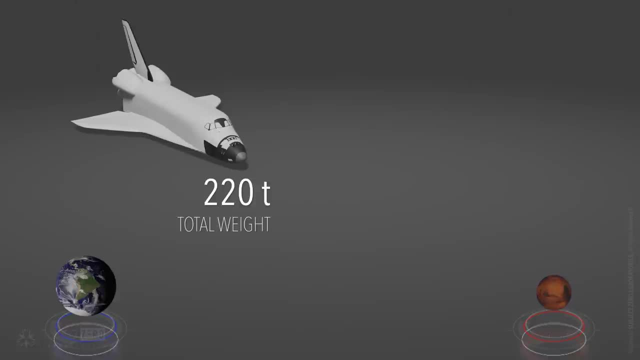 This will give enough room for astronauts to have a comfortable trip. If we were to use the space shuttle orbiter, we would have enough room for astronauts to have a comfortable trip. If we were to use a space shuttle orbiter, we would have enough room for astronauts to have a comfortable trip. If we were to use 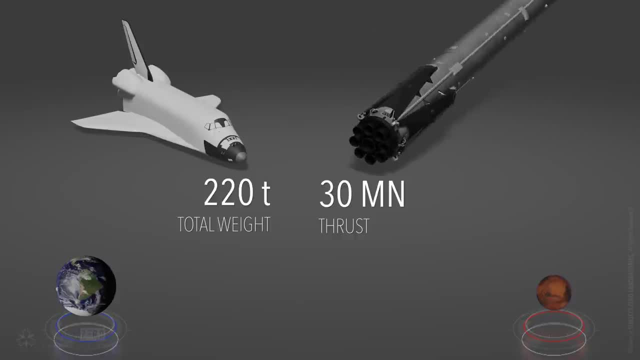 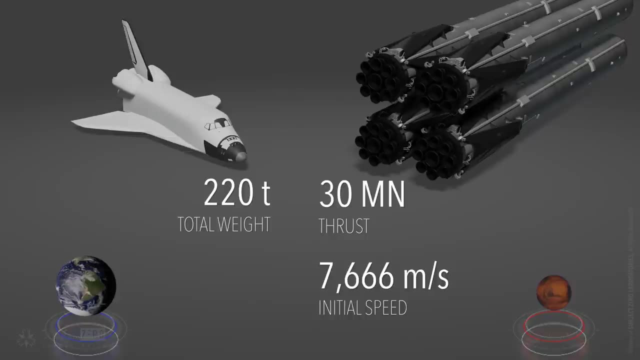 four chemical rockets delivering 30 million newtons of thrust, like Falcon 9, to propel the ship, and assuming it will be accelerated from the ISS orbit to its final velocity, the ship would generate 15.6 meters per second square of acceleration, whereby the end of its burn time 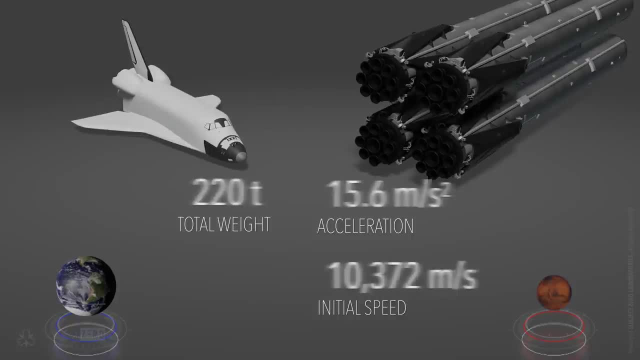 would achieve a final velocity of 10372 meters per second. With this speed, reaching Mars would happen in 125 days, or 4.6 billion days- Let's see what happens in 10 seconds. 4.2 months. It seems like a good choice, but there is a problem To reach that speed alone. 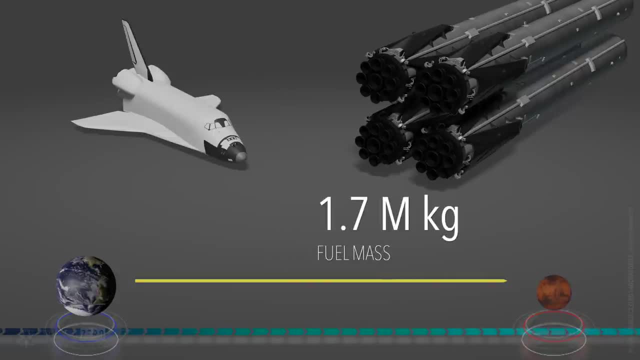 the total fuel mass is already 1.7 million kilograms. Making a very simple calculation, assuming that the same amount of fuel will be needed to decelerate the ship and travel back to Earth, we would need 7 million kilograms of fuel, That is, 31 times the mass of the ship. where 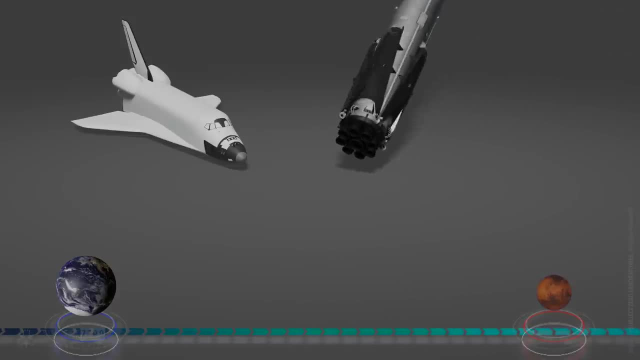 the astronauts are located Following the same logic for nuclear propulsion. the best proposed and tested nuclear core, the Phoebus 2A, gave an output of 930 kilonewtons with a flow rate of 120 kilograms per second. With 4 engines and 3.7 million newtons of thrust, our spaceship would 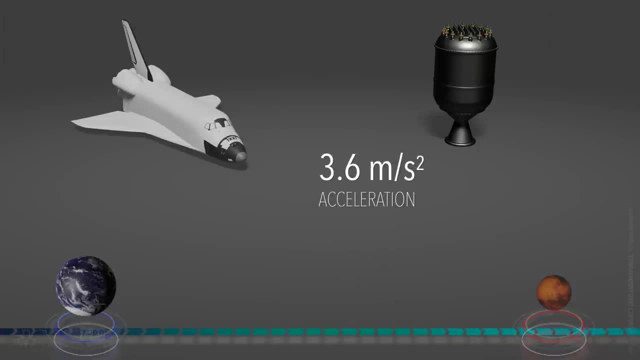 have an acceleration of 3.6 meters per second square. The difference here is that these rockets can burn fuel for longer times, Thousands of seconds. The best engine had a burn performance of 109 minutes. If we were to use just half of that time for our spaceship, we would get a final speed of 15,000. 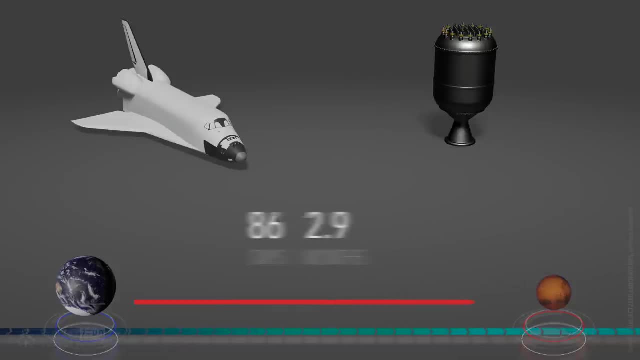 meters per second, which would make to Mars in only 3 months. with less than half the fuel, or 818 tons. Making the same assumptions as before, the total fuel needed would be only 3.2 million kilograms, Only 3.2 million kilograms.